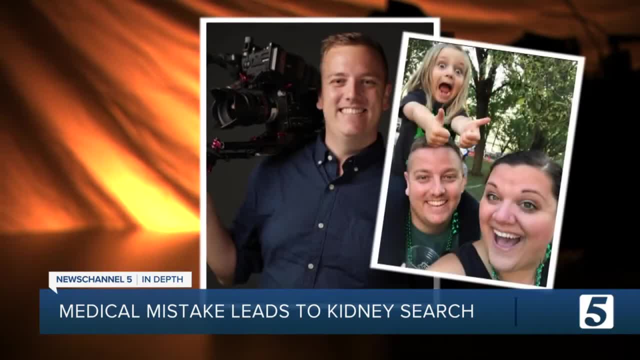 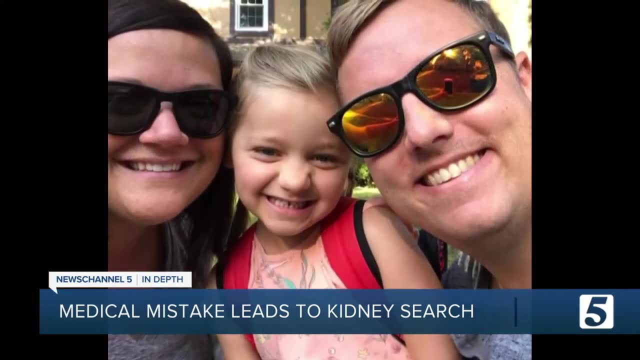 Now living in Kansas City, the talented photojournalist, husband and father. We're blessed to be parents of a five-year-old who- you know she's rambunctious and a very busy girl- Is also the owner of two failing kidneys. 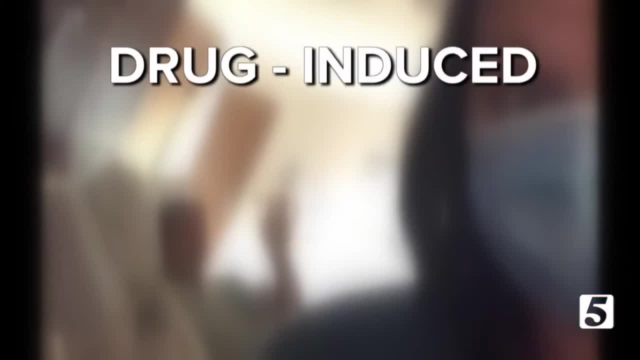 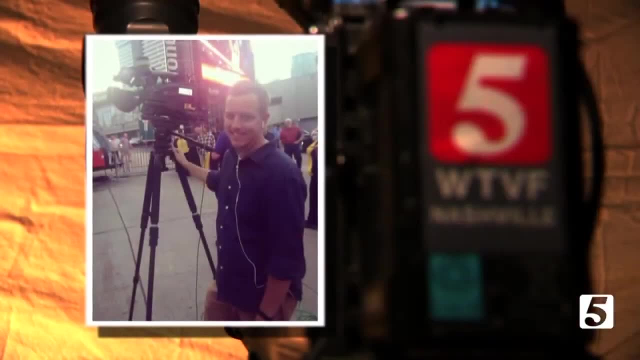 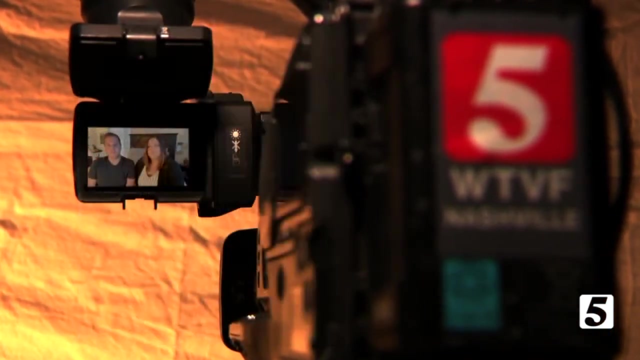 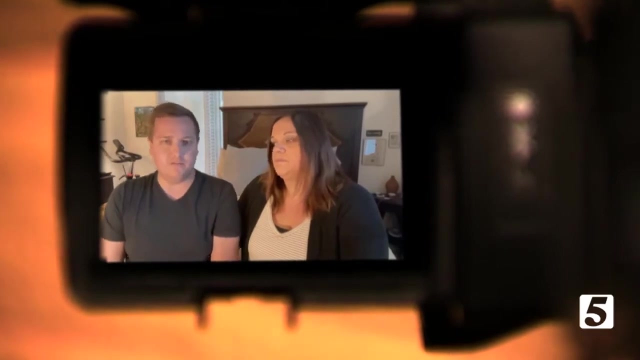 They determined to have this condition, called drug-induced interstitial nephritis. A doctor's mistake in treating his ulcerative colitis landed him in the hospital And, at 33 years old, news that changed his life: He needed a kidney transplant. The result of the biopsy basically discovered that I had lost at least 60% of my kidney function in both kidneys. 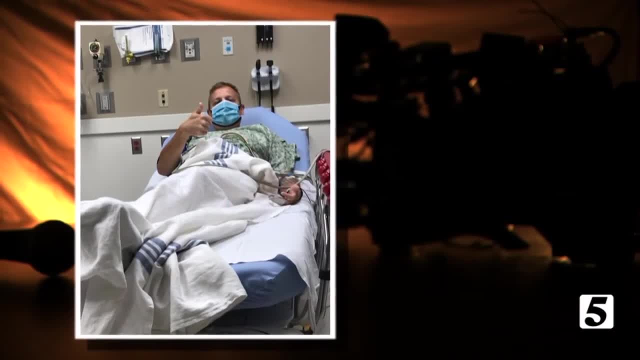 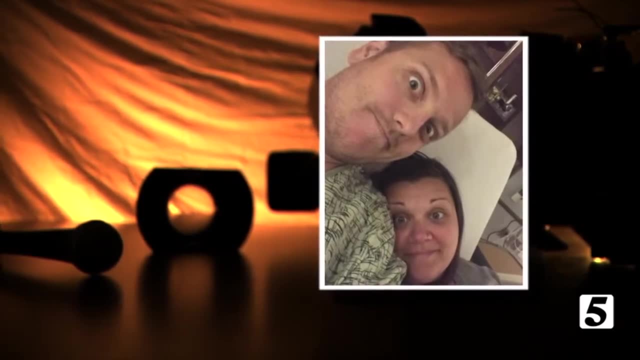 A revelation that could change a person's life. That could turn anyone bitter. I find that the two of us- we don't sit in that place very often of could have been prevented, shouldn't be here. No one will ever be held accountable. 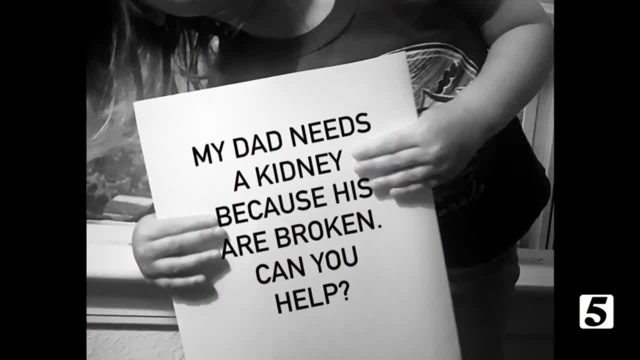 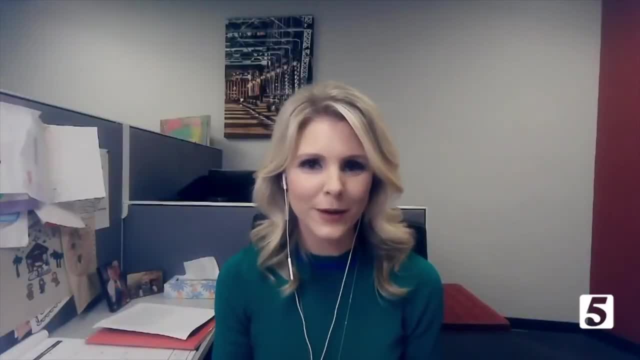 But for the Browns, it put them on a mission to find a living donor which will give Alex the best chance at life. Let's talk about asking for a kidney. That has to be weird. How do you go about even asking for a kidney in the first place? 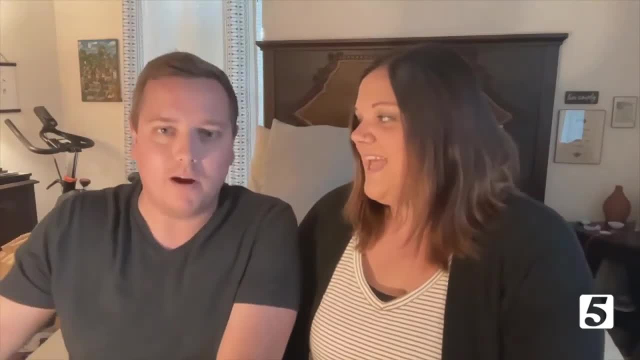 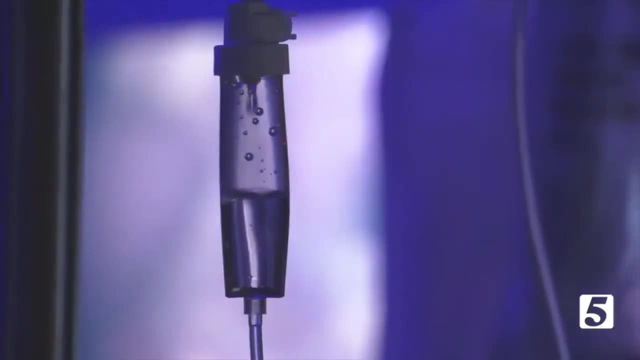 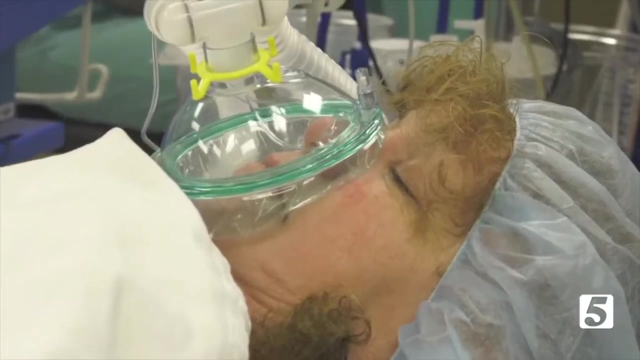 I have a hard time asking for somebody to give me 20 bucks. Kidney donations are the most common and successful among living donor transplants. A donor can be a family member, friend or even a stranger. Extensive medical testing is done beforehand to check for compatibility and overall health, all paid for by the recipient's insurance. 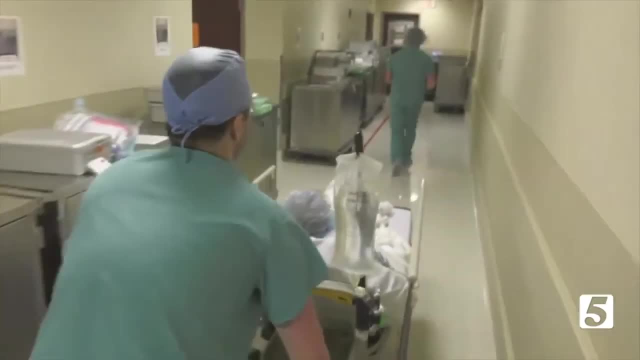 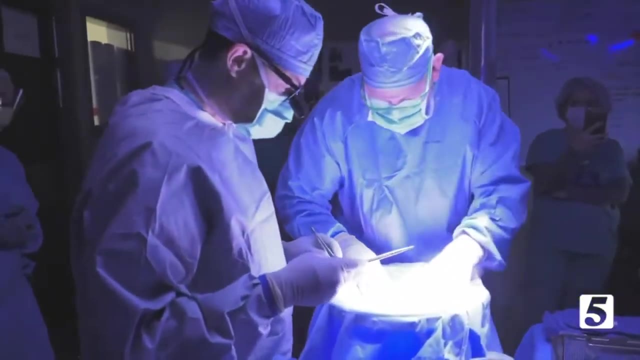 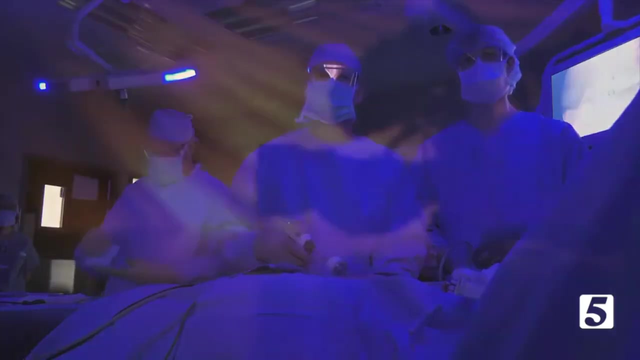 Patients spend, on average, three to five years waiting for a kidney from a deceased donor, But a living donor is the best option, as it allows recipients to live a longer, healthier life. But either way, it is a process that requires patience and living with uncertainty. 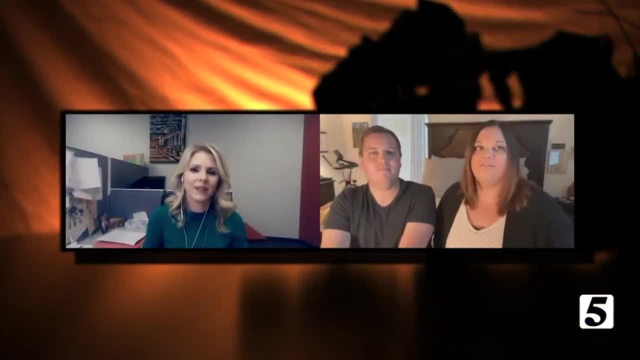 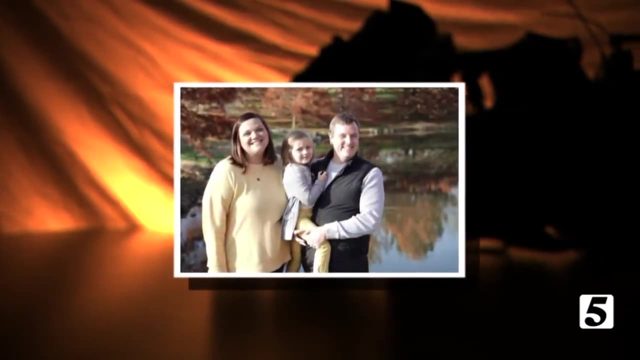 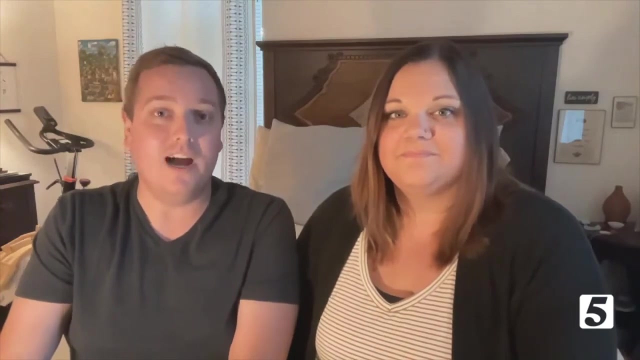 It really has changed every single thought that we have for our family, moving forward of what is best for what we have. right now, Two years since his diagnosis, Alex says he's doing okay. Right now I think I feel fine. but my doctors say, look, once you get a kidney, you realize how bad I've been feeling. 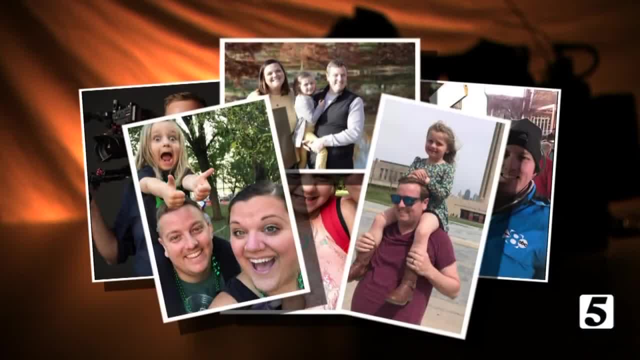 But there is no doubt this journey can be hard on the heart. Alex lives a life. Alex lives a life. I've happened to have those blue gut인가 Faith and dreams. God bless you. Holy, see you. God bless you.